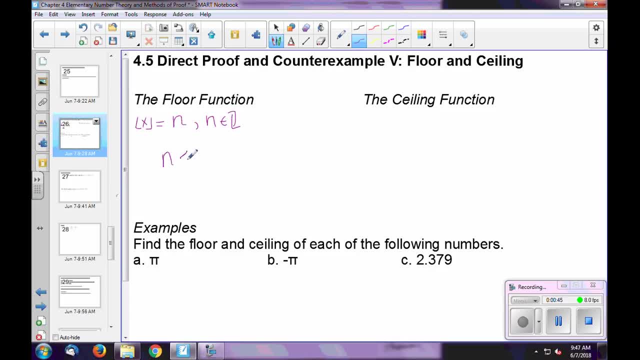 with the following requirement: n has to be less than or equal to x, but that has to be less than n plus one. So in other words, we're saying here that x, that real number, is bounded between an integer, n and n plus one, So those are consecutive integers On the other. 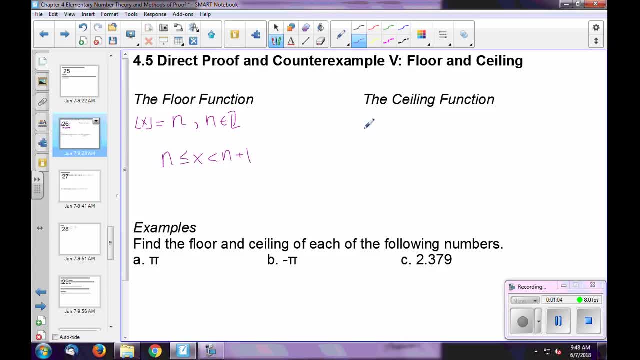 hand the ceiling function is going to take whatever your value is, whatever that real number is, and round it up to the next whole integer. Now this looks like the following: n minus one is our lower bound and then our upper bound is that value. 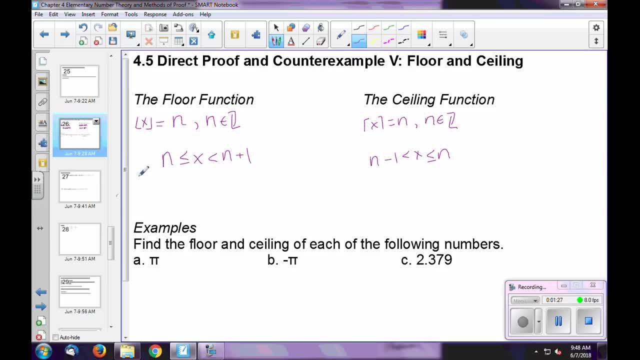 So you'll notice here what's the difference. The floor function is rounding things down, it's truncating them. So n is your lower bound, because that's what the floor function equals. On the other hand, with our ceiling function, where we're rounding up, n is our upper bound. So just a couple of. 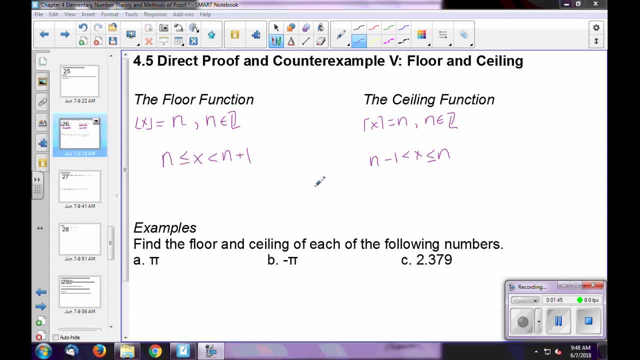 examples here, and something to be mindful of is that the decimals again are in some ways insignificant. it is really just saying: are you rounding this down, are you rounding this up? we can say that the floor of pi, in other words, if you're rounding pi down, would be equal to 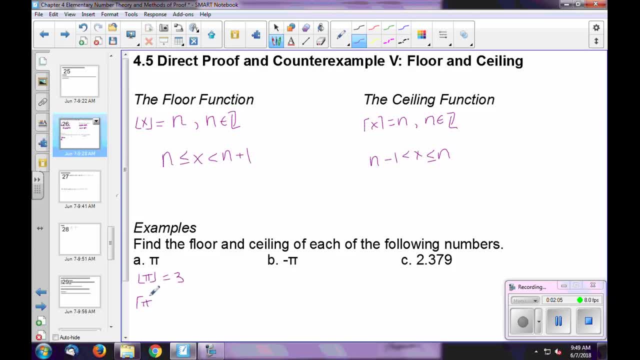 three, whereas the ceiling of pi we're rounding it up to equal to four. if you introduce a negative number, things get a little funny, but it's really not too bad. think about that for a second. the four of negative pi, so negative 3.14 and some stuff. if you round that down, it's actually going. 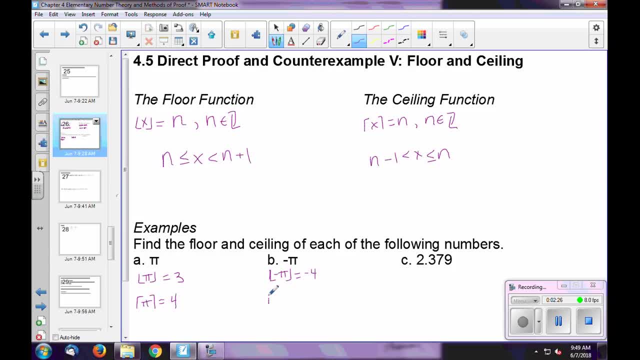 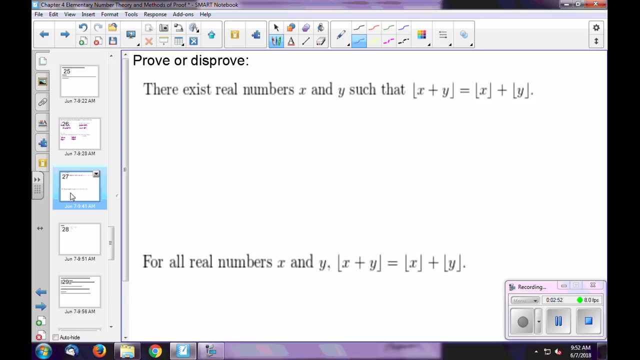 towards negative 4, whereas if you take the ceiling of negative pi and you round that up, you're rounding that up to negative 3 instead. let's take a look at a few examples pertaining to existence proofs. remember, with existence proofs, you only need to provide one case where this would 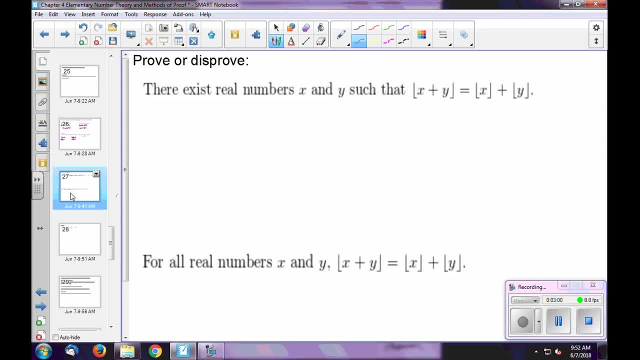 work. so if we're saying that there exists real numbers, x and y, such that the floor of x plus y is equal to the floor of x plus the floor of y, we only have to find one case where this would work out and bear in mind that. 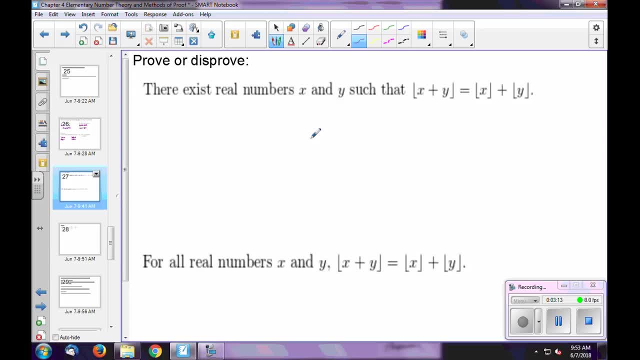 there can be more than one case, but you just have to show one time where it works and that means that the entire statement is true. so you can make this as simple or complicated as you want. keep it simple. let's see here, if we take something like i don't know, let's say let x equal 1.5. 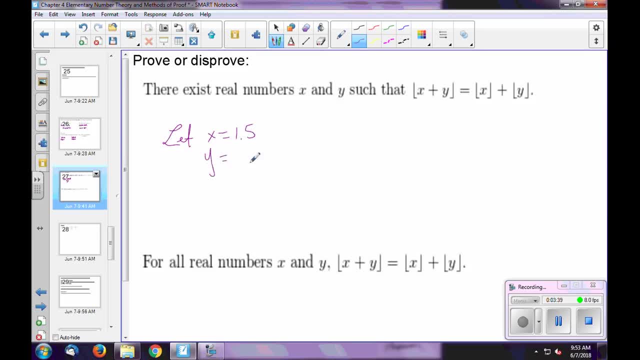 and y equal to 2, what would this give us? the floor of 1.5 plus 2? well, that's the floor of 3.5. we need to know: does that equal? this is where we check the floor of 1.5 plus the floor of 3.5. 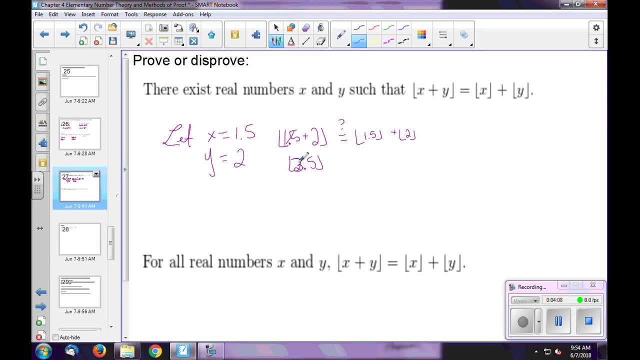 of 2.. 1.5 plus 2, let's see- gives us 3.5. the floor of 3.5 is 3. does that equal? the floor of 1.5 is 1 plus the floor of 2? choose already an integer, so it stays as is. there's no truncating or rounding. 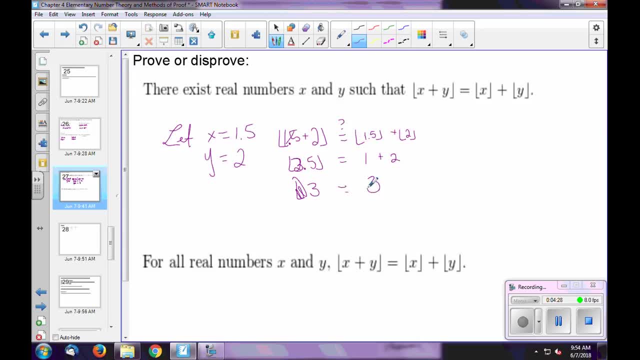 down. does three equal to three? yes, it does so. in this case, we have shown a case where this would be making the whole statement in fact true. now you can again get complicated with this if you wanted. you can use irrational numbers, make it fancy, but one of the conversations that i have with students in class is: well, it's nice if you. 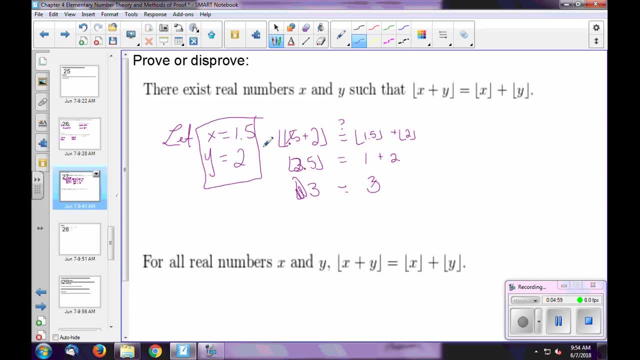 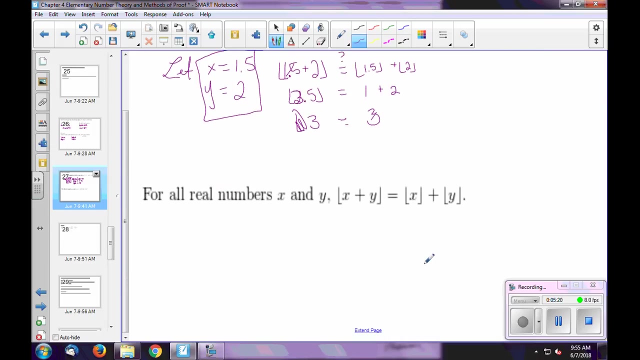 recognize that these work for fancy things like if you used, for example, pi and e, this would also work out, but there is no trying in언s. Let's take a look at this next one here, for all real numbers, x and y, the floor of x plus y is equal to the floor of x plus floor of y. 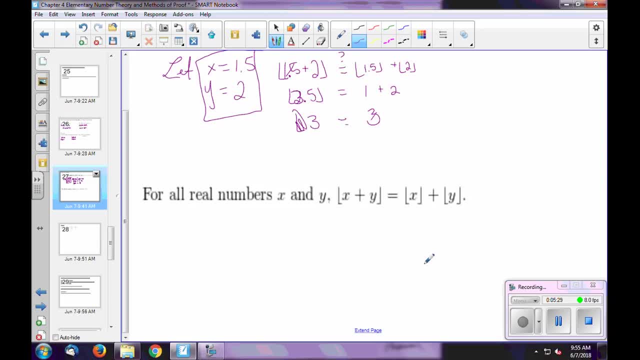 If you think about this, you should recognize very quickly that this is in fact, false. we're saying that this for all real numbers and it's not necessarily going to be the case. something you have to be careful of is when you add these two values together: x. 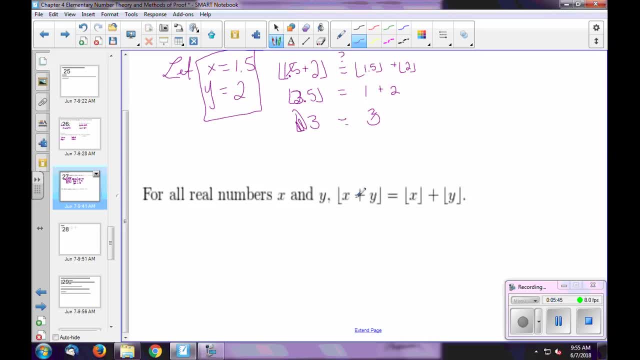 plus y. if that gives you a whole number, your floor is actually going to be very different than what it would be if you took the floor of those values separately. so again, pick anything. essentially that will make the sum in here equal to a whole number, but these are not whole numbers. so in this case, 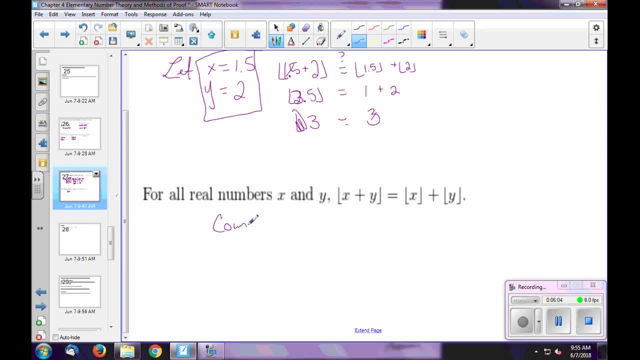 let's do a counterexample. remember, to disprove this we have to provide a counterexample. so let's say: let x equal 3 4ths, y can equal to 1 half. so we have then the floor of 3 fourths plus 1 half. and we're checking: does that equal the? 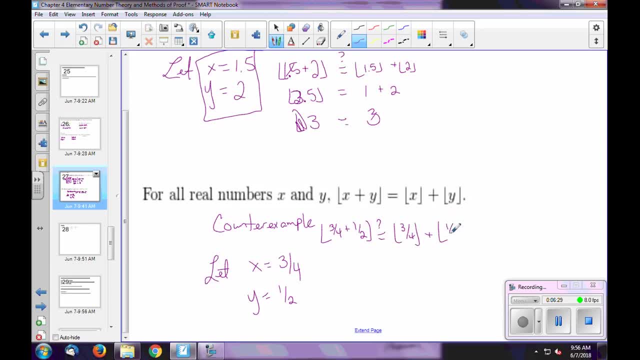 floor of 3 fourths plus the floor of 1 half. well, the floor of 1 half is equal to the floor of 1 half. so it's equal to the floor of 1 half. floor of each of these is going to be 0, since they're both smaller than 1, but 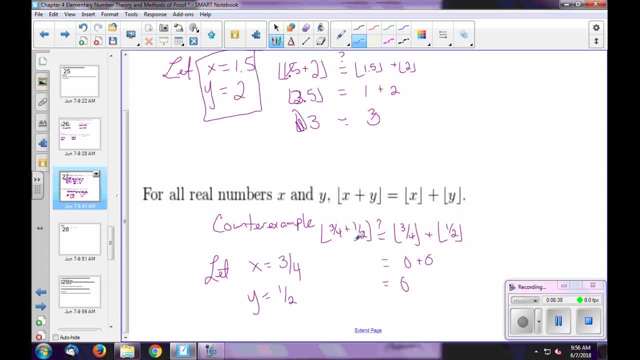 greater than 0. this, however, is the floor of 5 fourths, which is now greater than 1 but less than 2, so the floor of this is equal to 1, and, being that 1 does not equal to 0, we've provided our solid counterexample. let's take a look at one. 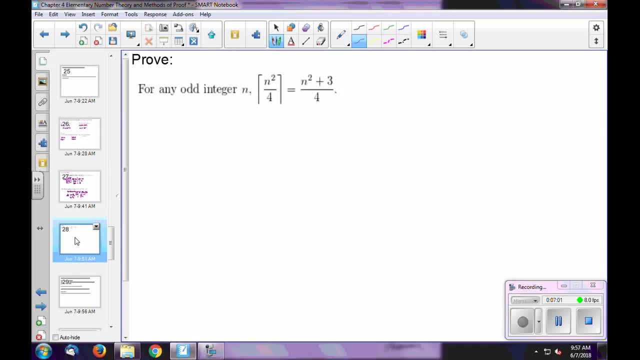 more example where we can use direct proof technique that involves a floor or ceiling function. now keep in mind the definitions we described on the first few minutes of this video. is we defined the floor and ceiling function using inequalities. so think about it in that way, because you'll probably have to. 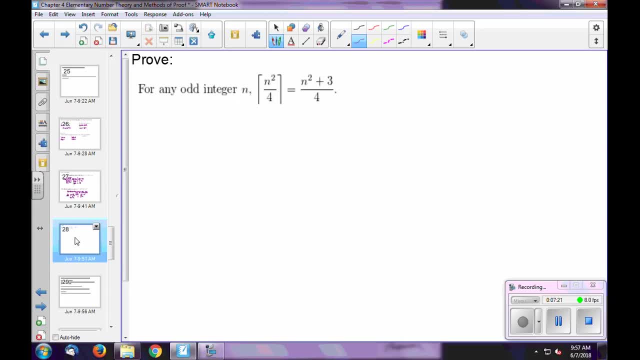 reference back to those definitions. when we teach direct proof, we talk about there always being some type of statement at the beginning. you know you're giving your hypotheses what's available, you manipulate that in some way and usually you have to use definitions to expand this information. so let's take a few minutes here and 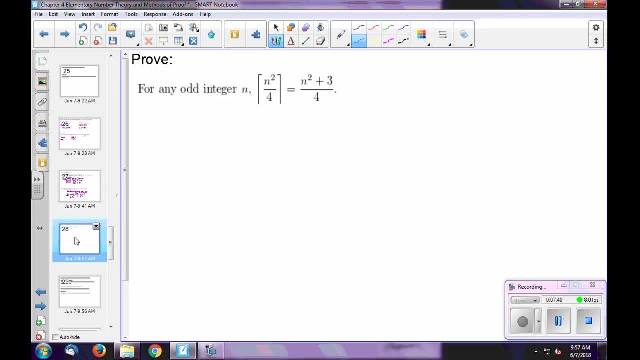 we're going to work through a proof using a ceiling function for any odd integer n. the ceiling of n squared over 4 is equal to n squared plus 3 over 4, so to prove this, it's going to start out just like any other proof that we've. 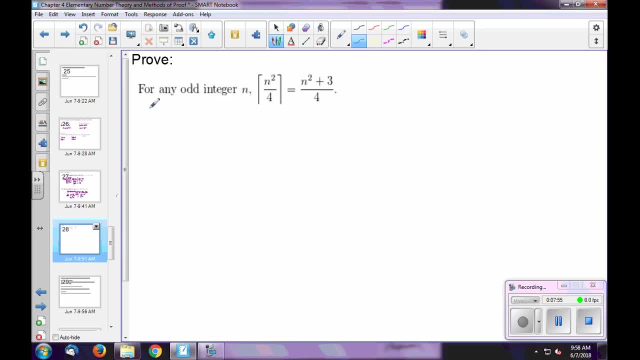 seen. there's nothing different right off the bat here. so for our proof, we start with the word proof, like any good proof starts with. we have this whole statement about any odd integer. that is our universal component of this universal conditional statement. that's incredibly important. so let's say that. 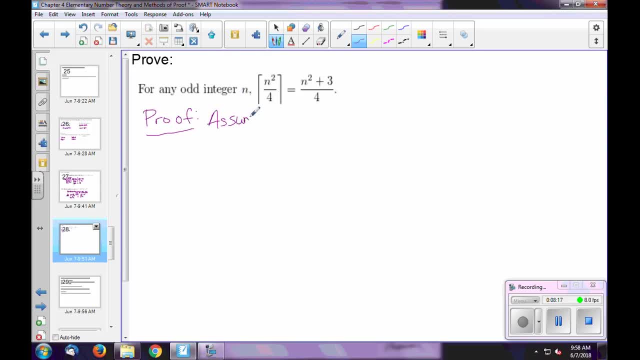 we assume- or let, however you want to phrase that assume- that n is an odd integer and we know that by the definition of odd, we can write that, as n is equal to 2 K plus 1 for some integer K, now, by substitution, we can replace n in each side of this and again, we're going to, we're going to work. 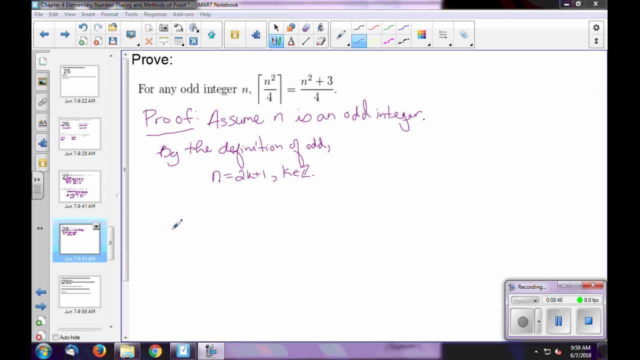 through this one step at a time. so take your ceiling function. here we know that n squared over 4, four on the left hand side, is going to now be the ceiling of 2 K plus 1 squared over 4, and something I've forgotten to write here. don't forget to justify that. 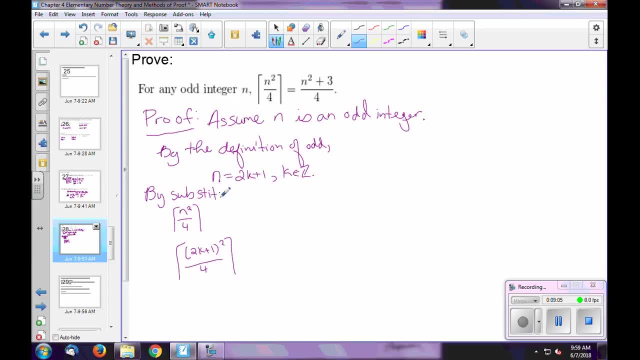 by substitution. this is equal to n squared plus 3 over 4. and then, on the right-hand side, do the same substitution there: 2 K plus 1 squared plus three, all over four. okay, so from here it's just going to be some manipulation we're going to do left hand side. 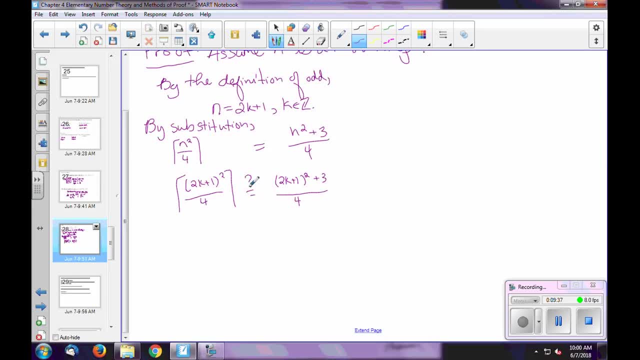 right hand side and we're trying to verify are these things still equivalent to one another? so take a few moments and expand this out here. for the sake of keeping this video from being excessively long. i keep pausing to write out the expansions. this is where you'd use your algebra. 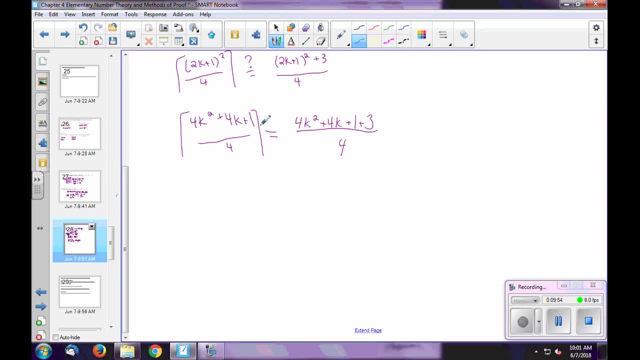 rate techniques. so if you're not sure where this is coming from, then either ask your instructor for help or look back in your old algebra notes from what you've done in the past. okay, so we can see how this expands using our algebra skills and we're going to combine like terms here. still on, 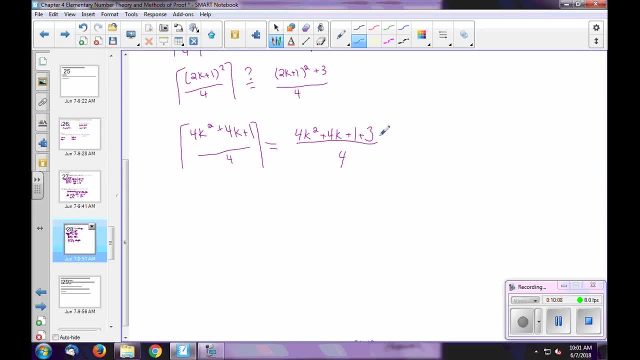 the right. so you have plus 1, plus 3 is going to be 4.. on the left hand side, it may not seem intuitive to do this, but anytime you're dividing, you're trying to figure out what would be an integer and what's not going to be an integer, because everything that you 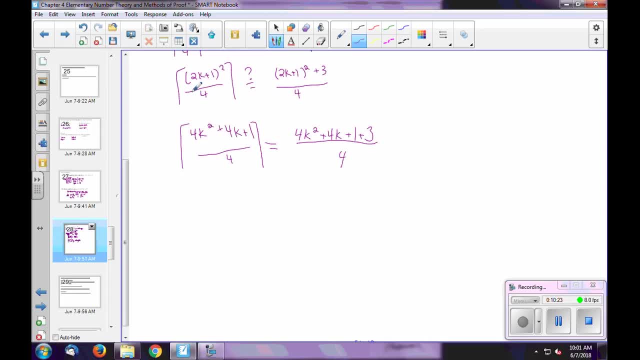 do is going to be an integer and what's not going to be an integer? because everything that you do here is pertaining to the answer being an integer of some kind. remember it's in this case, it's a ceiling function. so we're going to be rounding up, so what does this part look like? you're going to 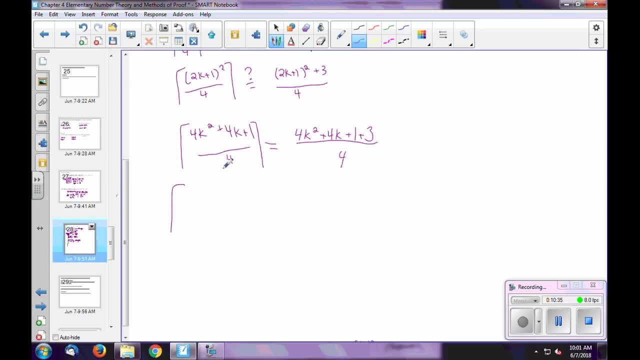 break this up. this is 4k squared over 4. well, that's k squared plus 4k over 4. it's going to be just k plus 1 over 4 is 1- 4. there's nothing we can do to simplify that and again, you'll leave that part as is okay. 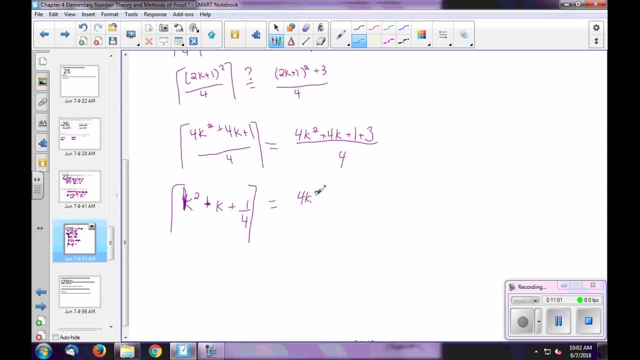 on the right hand side- i'm going to clean this up a bit- you have 4k squared plus 4k plus 4, all over 4, and we should notice that everything here is divisible by 4. so on the left hand- i'm sorry, the right hand side- you now have k squared plus k plus one. how can we get the left hand? 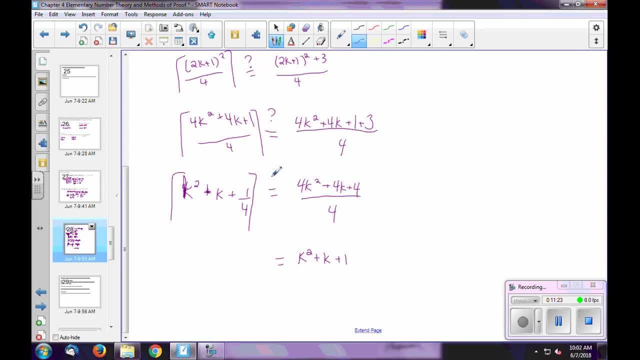 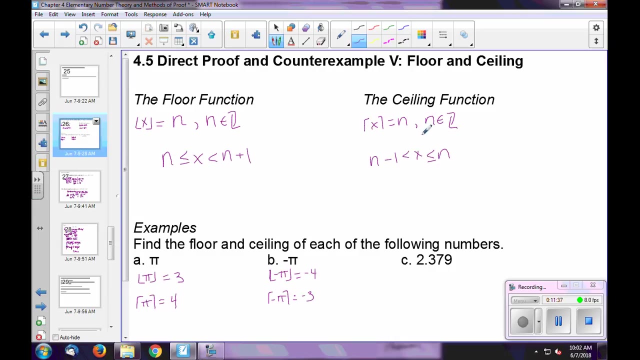 side to look something like this. we're still trying to verify: are these things all equal to one another? well, this is where we have to come up using our definition of a ceiling function to try and manipulate this a little bit. so if we flip back to our definition of a ceiling function, 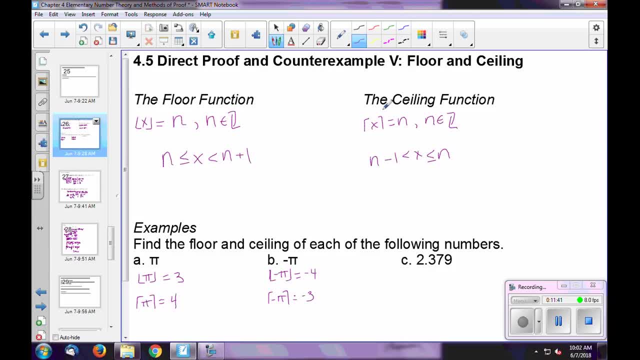 when you take the ceiling of something, for example, when you take the ceiling of k squared plus k plus 1, 4, you need to figure out what your lower bound would be and what your upper bound would be. so, whether you do this off to the side or not, say perhaps even just right below it, 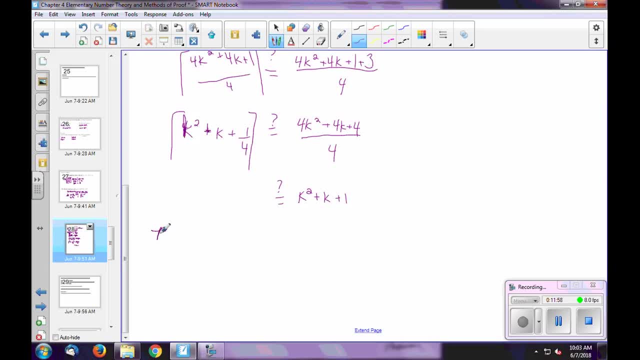 and say by the definition of ceiling, ceiling function, i should say: remember this is bound in the center: k squared plus k plus k squared plus k squared plus k squared plus one-fourth k squared, being that we defined k to be an integer is also an integer. k is an integer when you add: 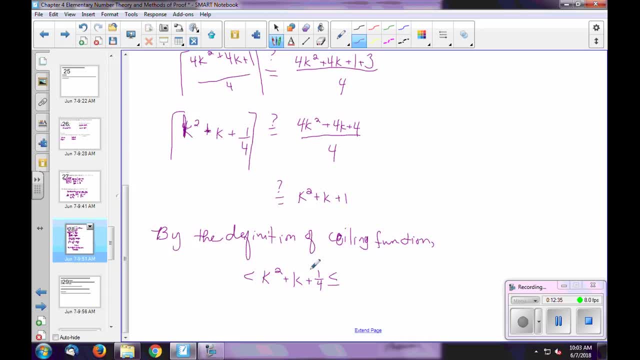 two integers together you get an integer. an integer plus a rational number is going to be rational. so if you have an integer and this rational component and it's a ceiling function and you were to round it up, you would take that then to k squared plus k plus one, because that would make it the next whole. 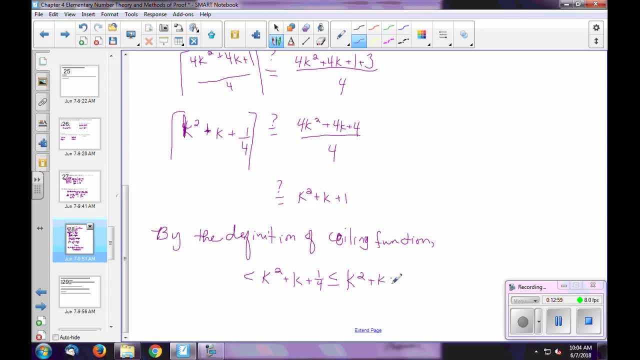 integer. on the other hand, if you were to round this down, one-fourth truncates off, and you're left with k squared plus k. remember, though, how it's defined: it's equal to n, and n is the right-hand side of this inequality. so how does this all piece to you? 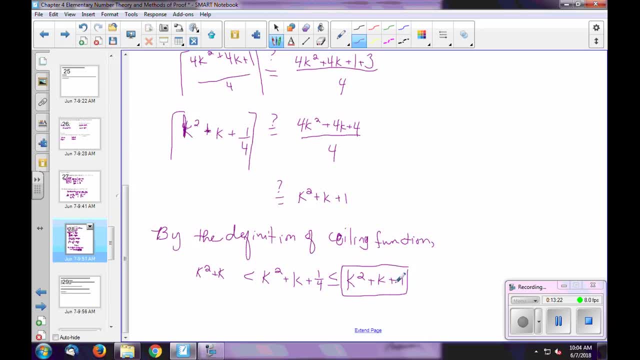 so how does this all piece to you? it's all pieces back together because we substitute one last time this statement up here. this ceiling function is directly equivalent to what we've done down here, so that part was just for illustrative purposes. we're going to get: 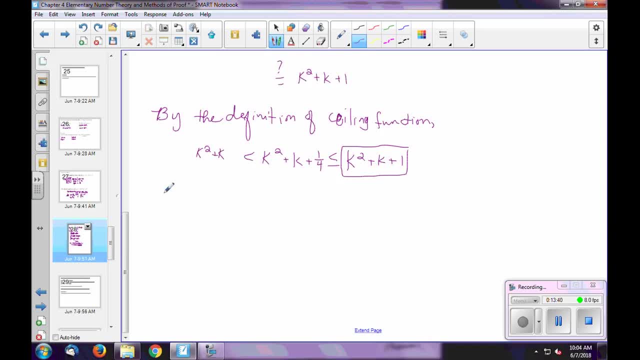 rid of that through our proof. but one last statement to make. by substitution again, we've shown that K squared plus K plus 1 is in fact equal to K squared plus K plus 1. it's exactly what we were after. so therefore, for all odd integers, 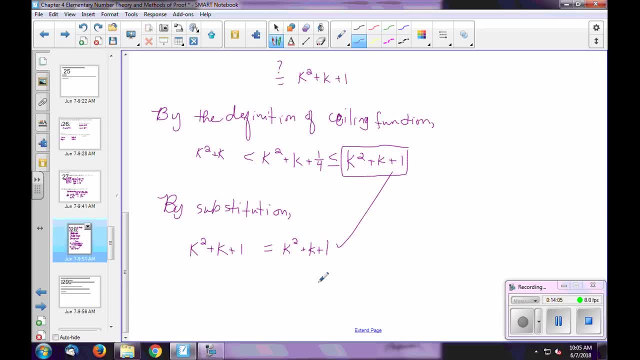 the ceiling of N squared over 4 is equal to N squared plus 3 over 4. once you have that written out, remember, you restate to wrap up your proof, and then you either put your filled-in box or you can use QED, so whichever style is becoming comfortable.